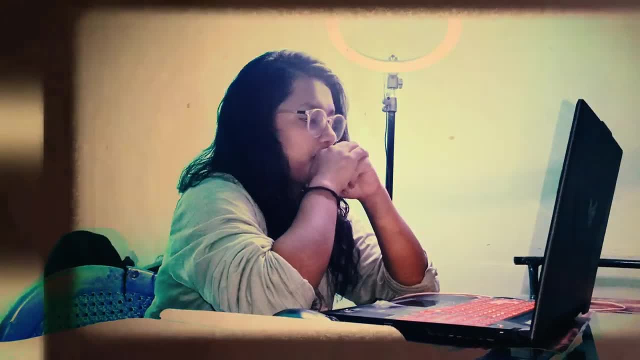 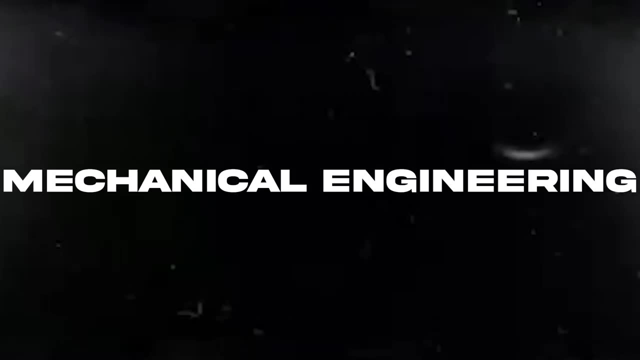 7th December 2021.. I was waiting for my CSAB counselling final round result. Before that, in Jhosa till round 6, I was allotted Mechanical Engineering at NIT Roorkela And I got a bit anxious. kyunki yaar kaafi senior, se baat karne ke baad ye sunne me aaya tha. 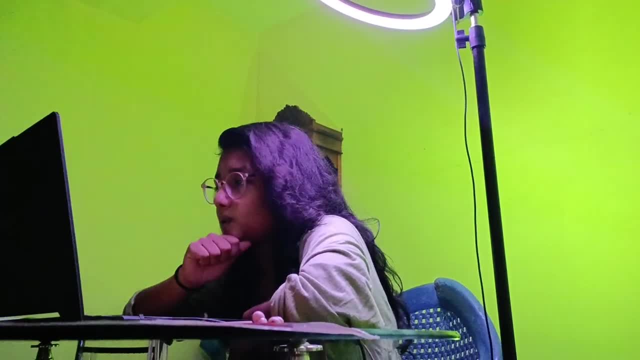 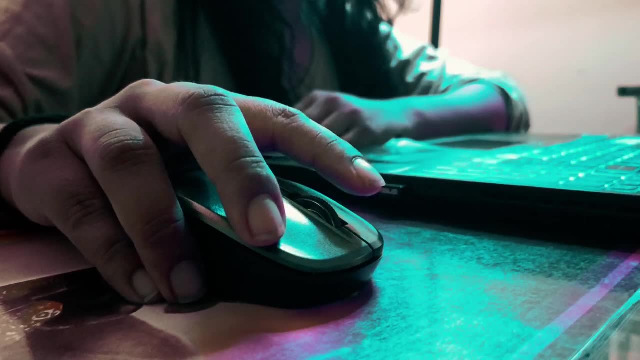 ke mechanical engineering. me kaafi physics aati hai, And I was weak in physics. yes, Ishliya, I applied for CSAB And finally the CSAB results came out and what I saw on screen was Institute named Vishweshwarya National Institute of Technology. 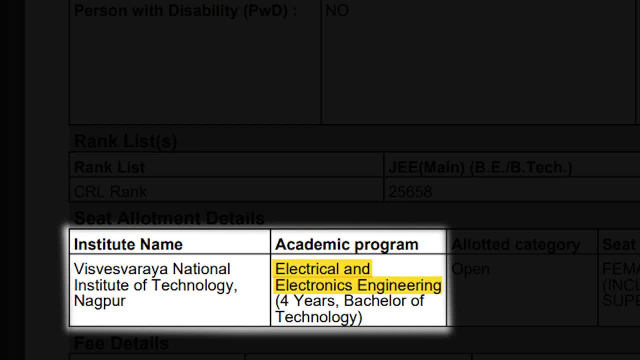 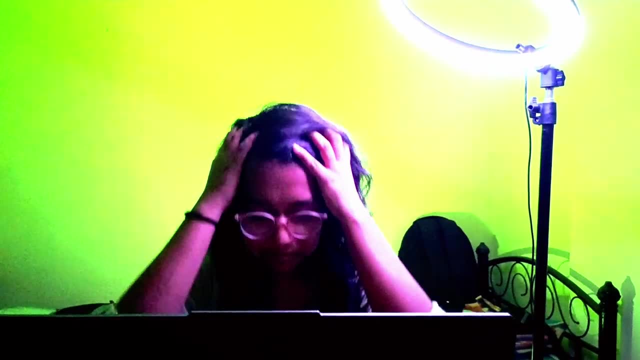 Nagpur Academic Program, Electrical and Electronics Engineering, 4 years Bachelor of Technology. I was a little shocked, as it was unexpected, and of course, why not? as I was the branch closer Ab mai raheti hu Guwahati mein aur college mila tha mujhe Nagpur mein. 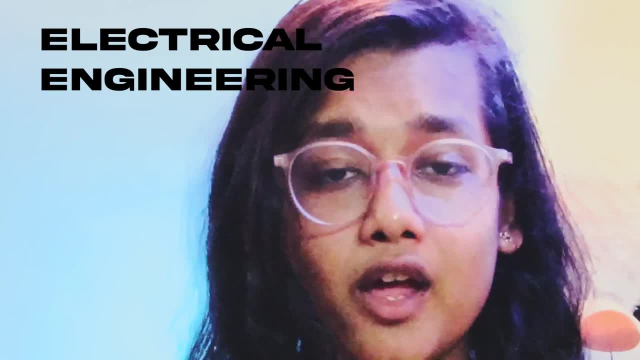 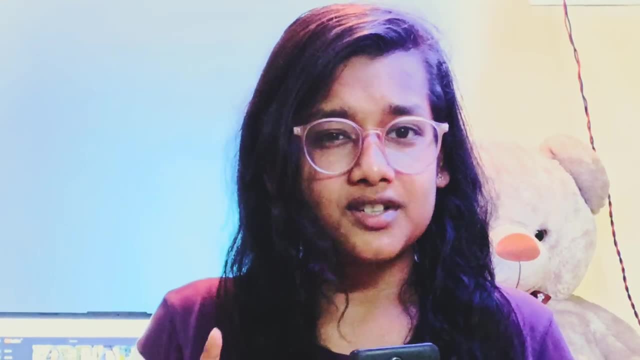 Aur upar se branch kaunsi Electrical Engineering, which is known for being one of the toughest engineering programs. To yaar tab meri gande wale lag gaye, the but shayad tab mujhe realize nahi hua. 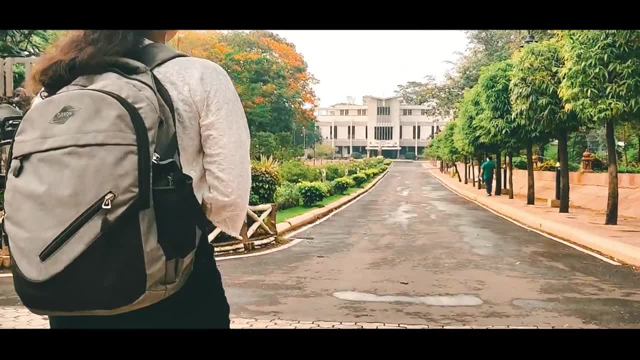 Bas ye socha tha, college jaake kuch na kuch jugaad hoi jaega hair hu huirما ki hu aakhir hum bhi to gonna be engineers hi hai Ab first year to mast haraam se online nikal gaya tha. 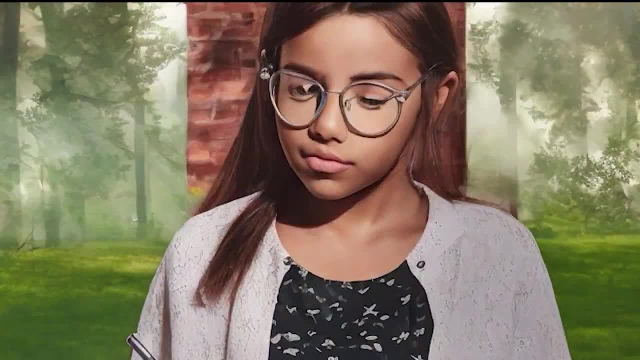 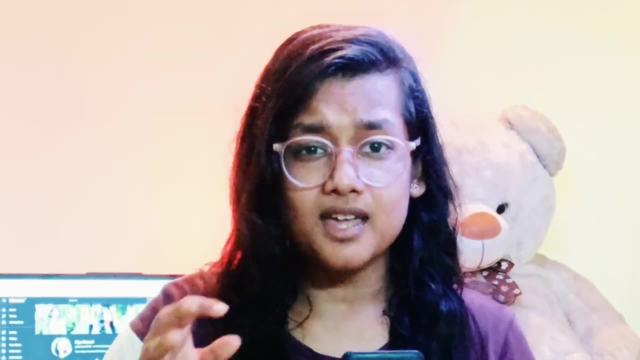 achchi gaha se CGPA bhi aa gaya thi aur phat na bhi ni pada tha. But haan, itna mind me zarur tha, ki coding to paralleli karni padhegi. Kiki, yaar, meri branch TRIPLE-E, me ek bhi coding ka course nahi hone wala tha. 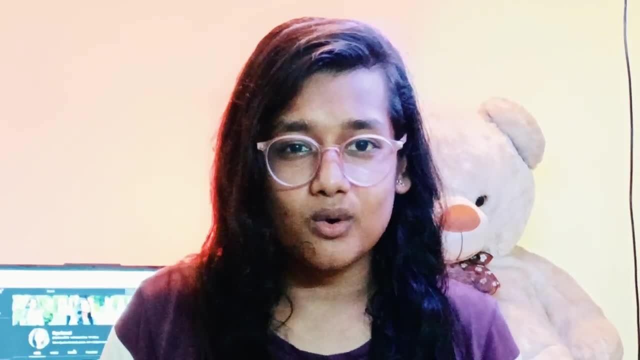 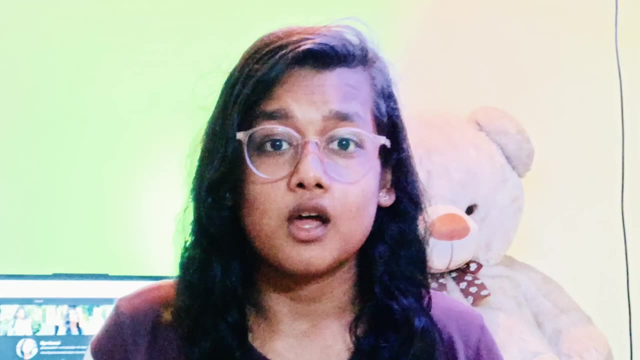 except for some optional courses. But yaar itna mind me zarur tha ki coding to paralleli karni padhegi courses. and now how do you do college courses? everyone knows that YouTube zindabad. now, in the first year I heard this from everyone: dude, do coding, you will get a good package. 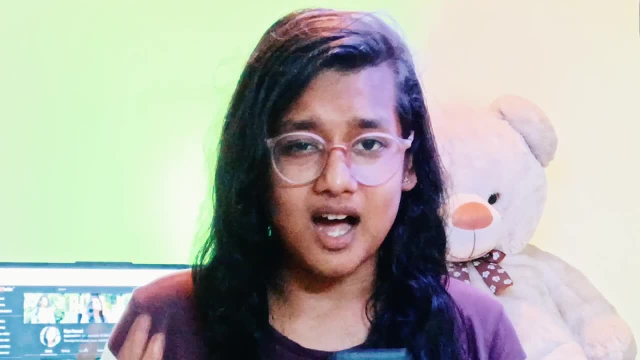 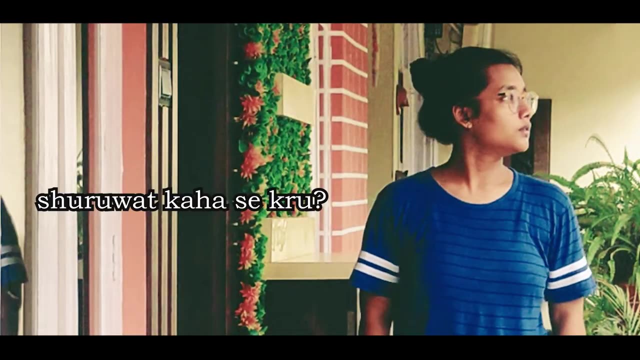 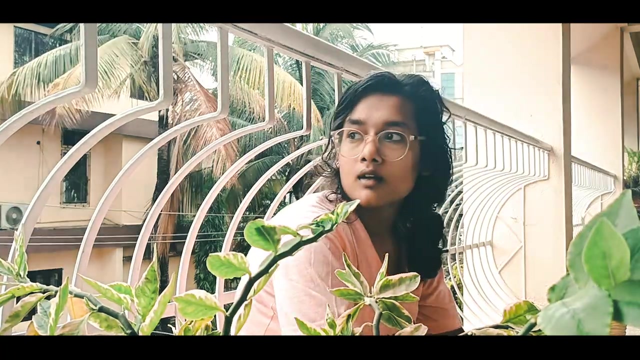 and one reason was also that there was no interest in online. so, of course, at the end, I had to do something at home, but I couldn't understand where to start. Too many thoughts to think deeply, too many thoughts to be sweeping- yeah, oh, my god. 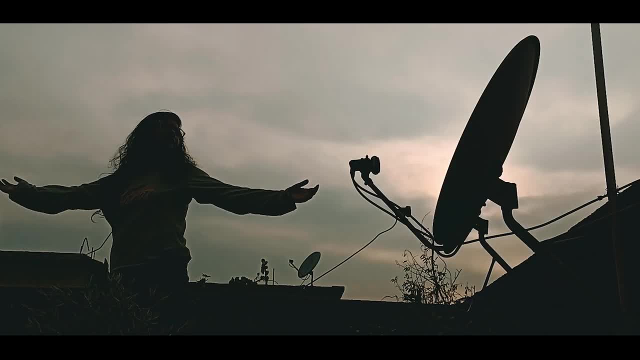 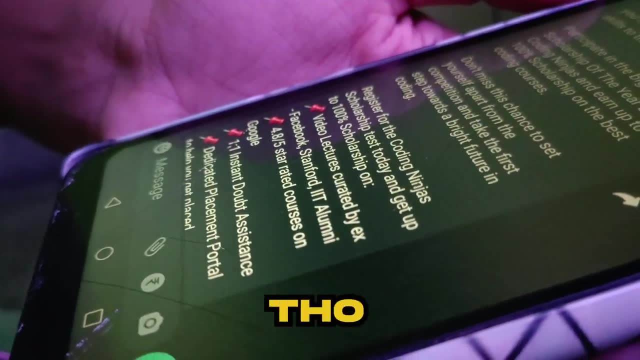 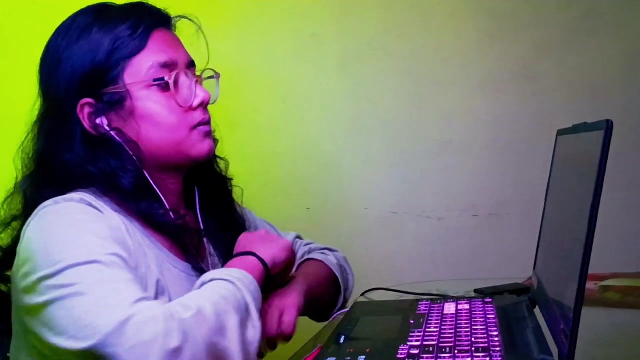 I'm not eating. I feel so empty I'm receding. so one fine day a senior comes to our group and says: you know, give this coding ninjas a scholarship test. if it goes well, you will get a discount on their courses. so I thought let's give it now some math aptitude questions. 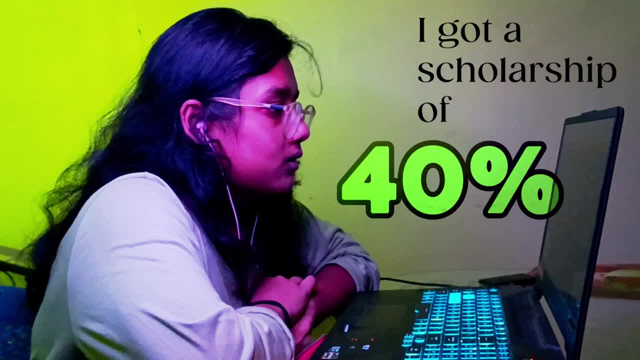 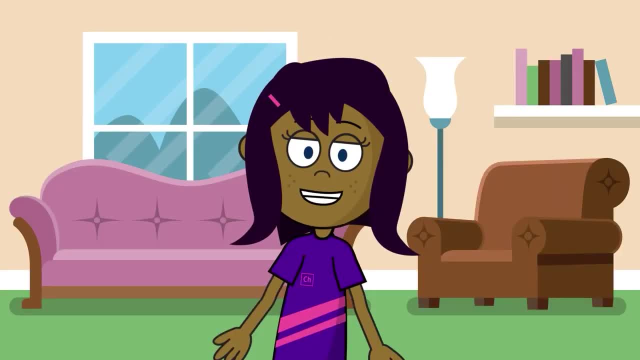 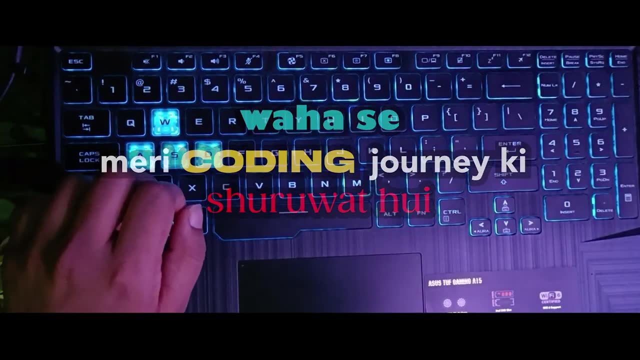 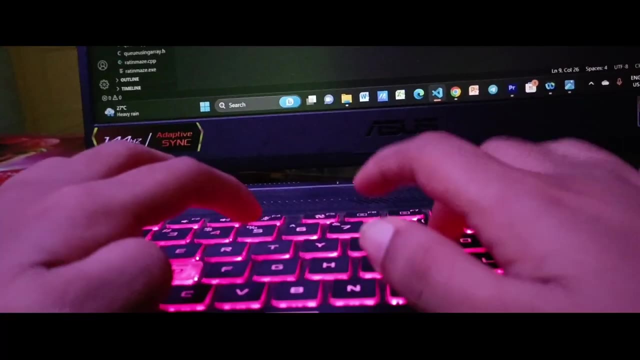 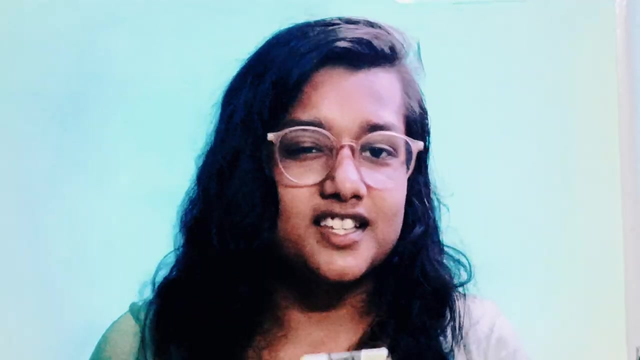 let's give a course. at least I would give a start to it. so I made dad happy a bit and then I took the C++ and DSA course. so that's where my coding journey started. As soon as the second year came, I started to have an interest in coding, and this realization 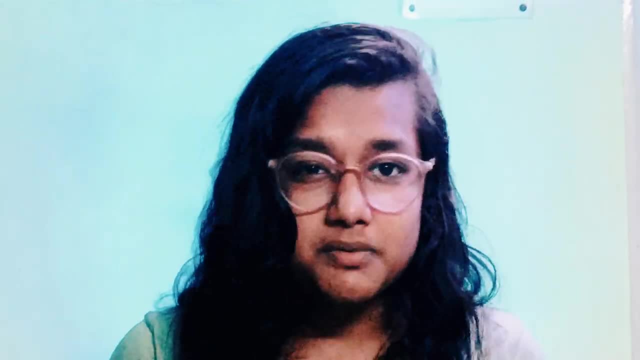 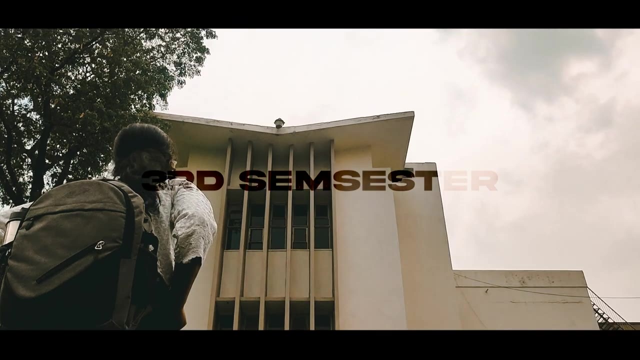 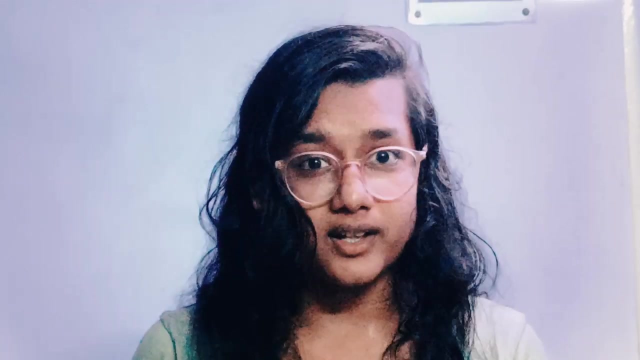 It would be much, much better if I was in CSE. My second year of college was offline, ie from my 3rd semester I had a feeling that I would have to pay attention to academics because the core courses of my branch had started, which were really bad. 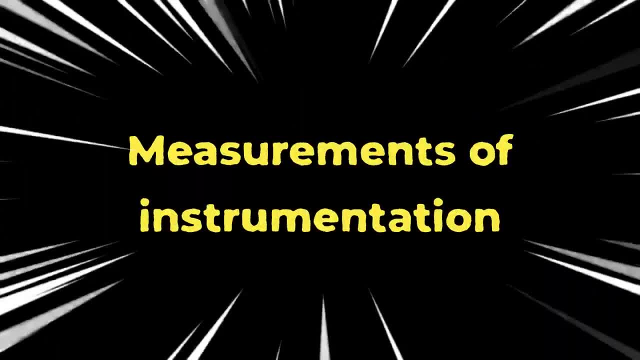 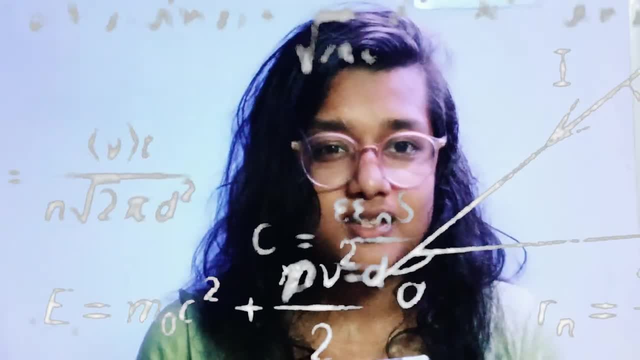 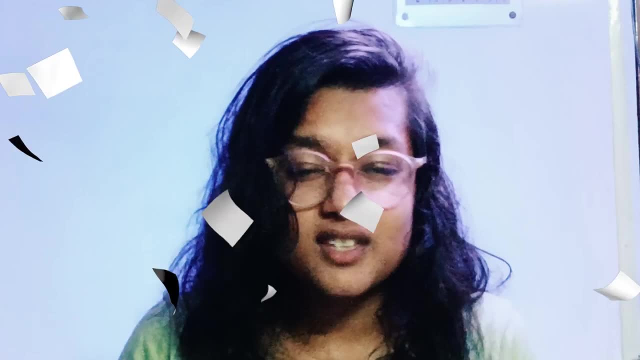 Elements of Electromagnetics, Measurements of Instrumentation, Network Theory. so many scary names, so many big derivations, so many useless calculations which are literally not even from a scientific calculator, 200 pages of PDFs and so many great professors. 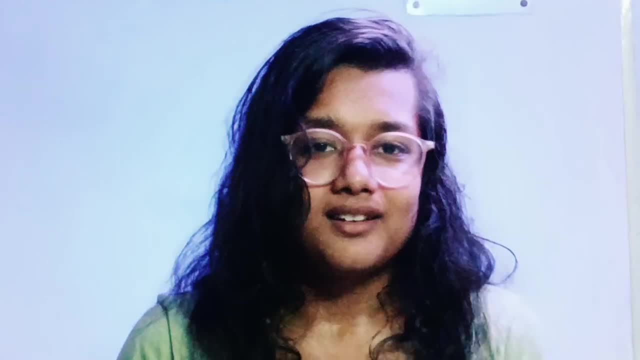 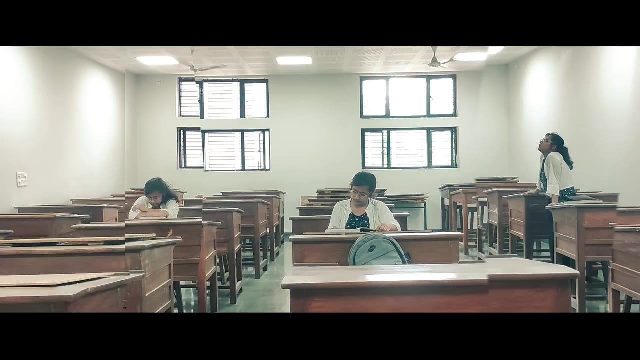 I mean, you know what I mean. I literally thought: what is all this? What will happen after studying? I mean, what is going to be useful in my life? Just get into the rat race, take the exam so that I get a good CGP. 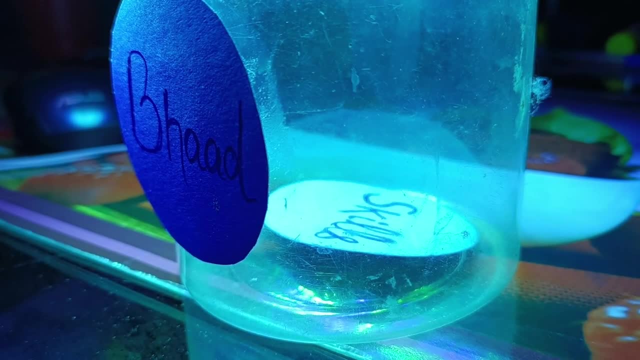 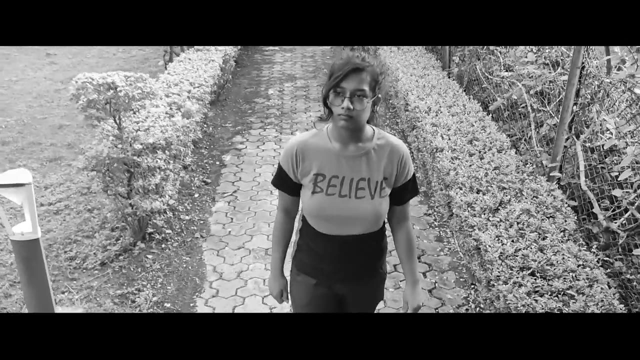 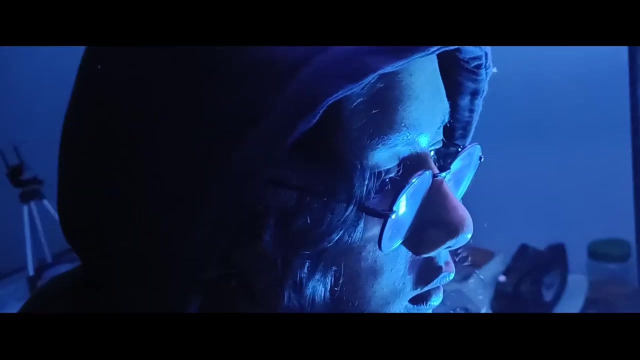 At least my skills went to hell. Seriously, all this was very frustrating, Where people were focusing on their studies and increasing their CGP while I was doing the things I was most passionate about. Sometimes I used to feel that I devote most of my time to coding. 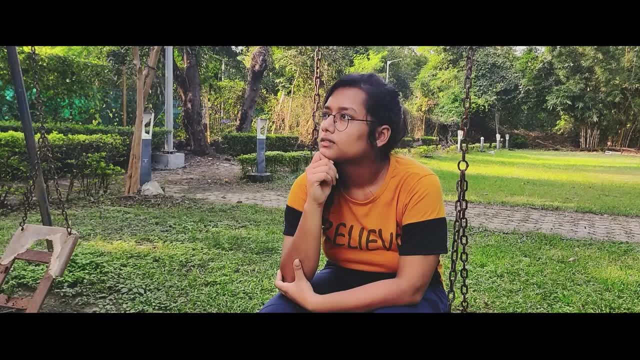 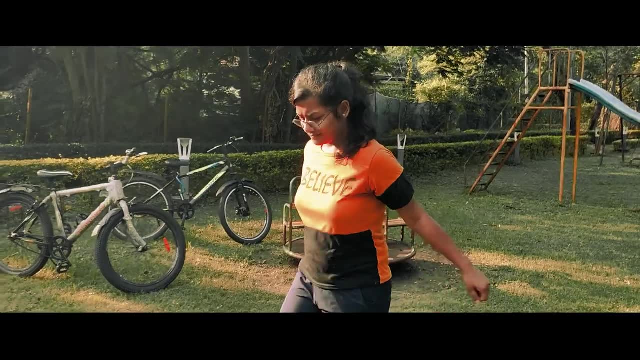 so that I can get a good job. And then I used to remember: no man, video editing and filmmaking also have their own fun. How can I leave that alone? And then one day I used to think I have been dancing since my childhood.